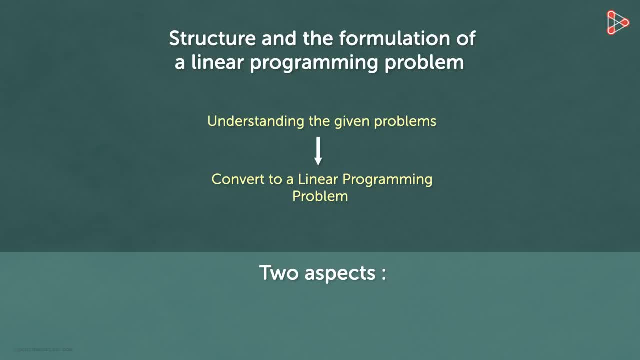 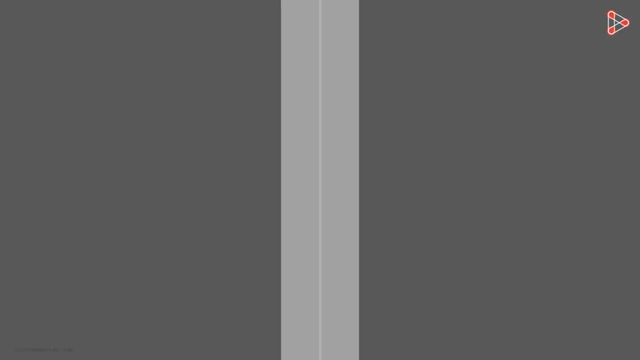 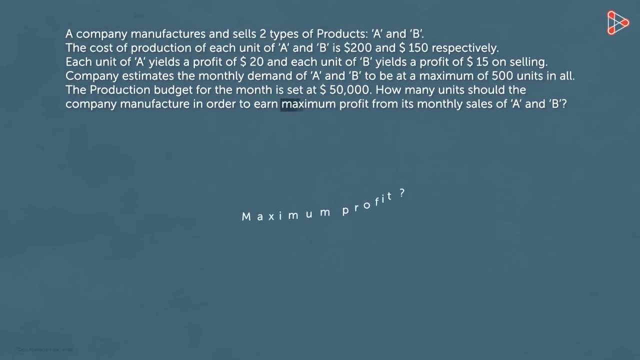 it. So there are two aspects here: The formulation part and then the solution part. Let's begin with the formulation of linear programming problems. Go through this example. We have to find the maximum profit the company can earn with the constraint. The constraint here is the maximum profit the company can earn with the constraint. 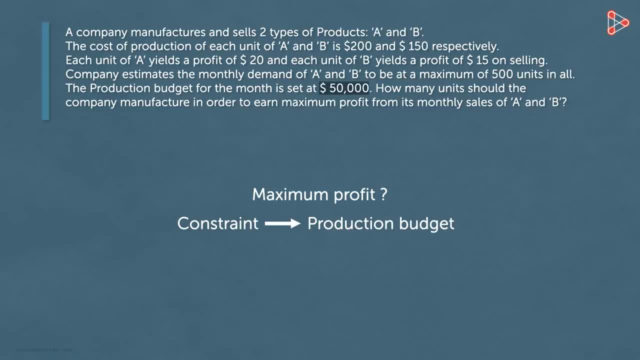 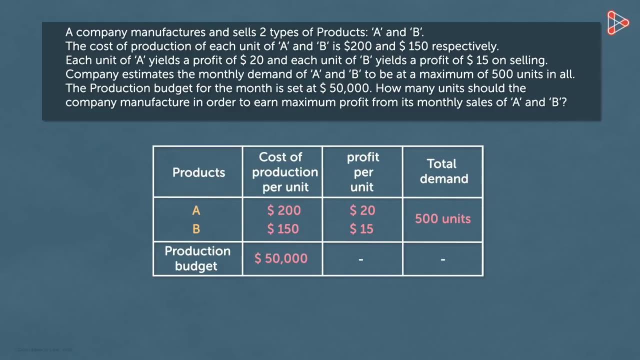 The constraint here is the production budget. But how do we approach this problem now? First, let's try to represent this problem in a tabular form. Can you give it a try? Here it is, Go through it. well, Note that we have to convert this problem into a linear programming problem. 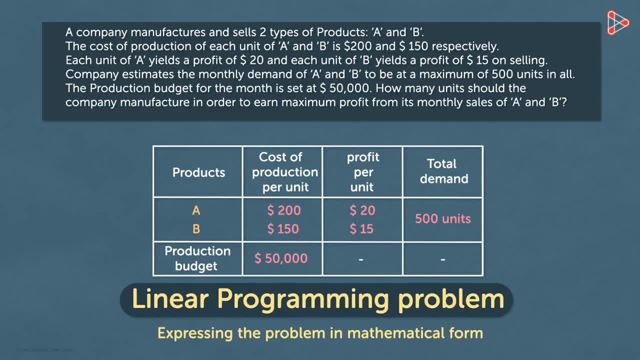 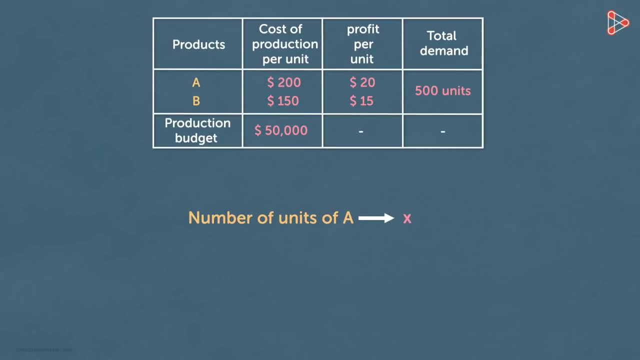 And how do we do that? By writing the given problem in the form of mathematical equations. Let's see how it works. First we need to write the number of units of product A to be X and the number of units of product B to be Y. 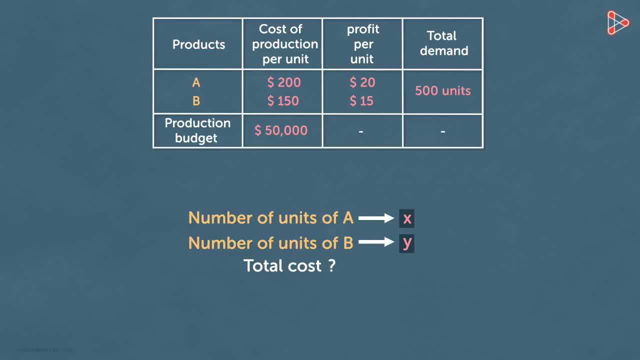 Now can you tell me the total cost to manufacture these many units of A and B respectively? Yes, it will be 200 times X and 150 times Y. We are talking about the total cost of manufacturing these many units of A and B respectively. 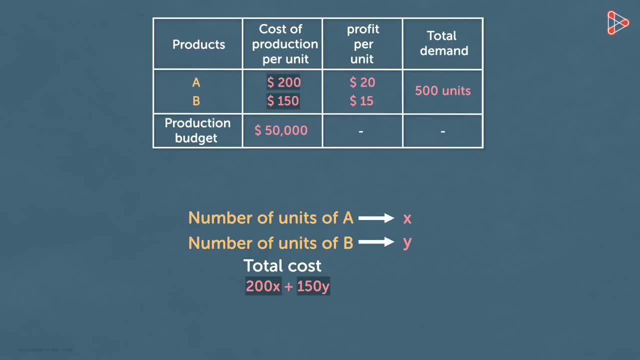 We are just multiplying the quantity with the price. Next let's look at the constraint. It says the production budget is $50,000.. That means the cost to be incurred should not exceed $50,000.. It can be less than or equal to $50,000. 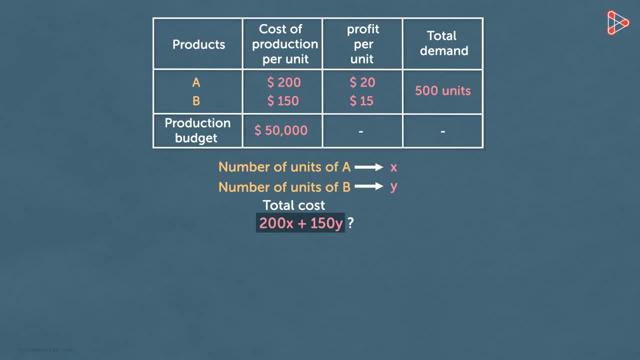 Can you write this constraint in the form of a mathematical expression? Here's the answer. This expression represents the budget. The cost to be incurred should not exceed $50,000.. It can be less than or equal to $50,000.. So the total cost is $50,000. 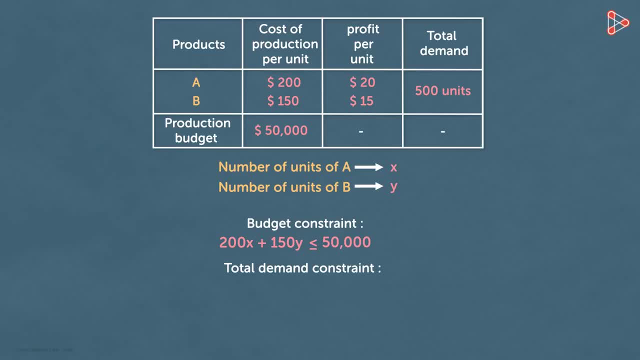 Now let's express the total demand of the two products in a similar manner. Give it a try. The combined monthly demand of the two products will not exceed 500 units. Therefore, we use the less than or equal to sign to write this expression. 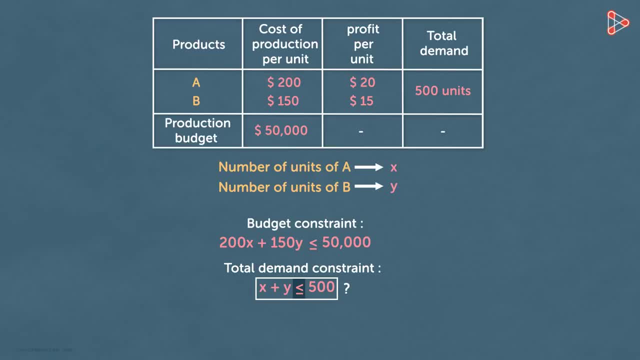 And which constraint does this expression represent? Yes, it represents the DEMAND CONSTRAINT of the given problem. This means if the company produces more than 500 units of products, A and B in all, it might not be able to sell them. Are there any other constraints in the problem? 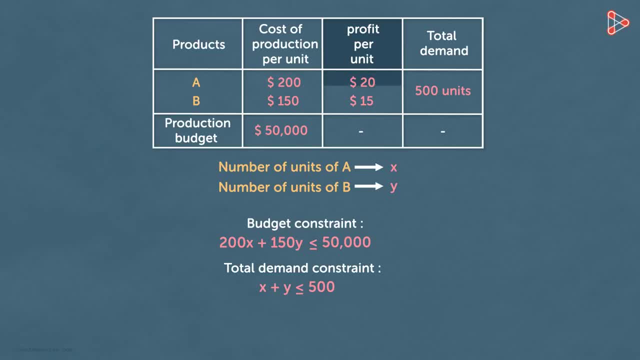 Not really. So let's look at the profit element of the two products. Can you tell me the objective of the company in this case? The company would like to sell its products A and B in such a mix that it yields maximum profit in a month. 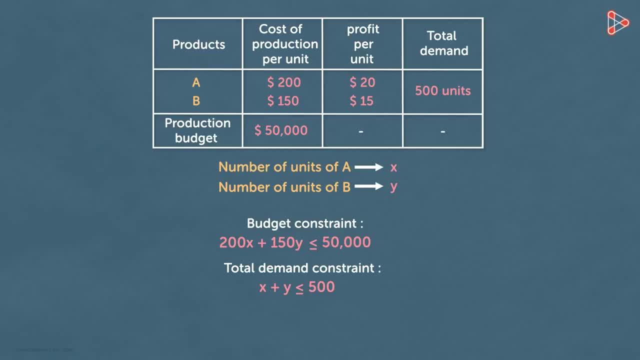 In simple words, the company would try to maximize the profit which it can yield by selling A and B. Now let Z denote the total profit for the month. Can you write the total profit in the form of mathematical expression? The total profit Z can be written as this: 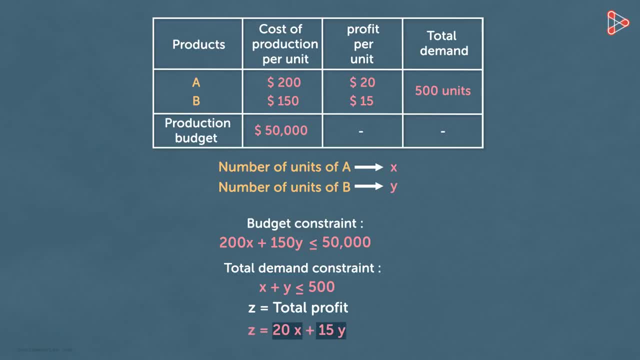 It's the product of the quantity and the profit per unit. With this we will write the objective function of this problem. The objective function in a linear programming problem is a mathematical expression of the ultimate goal. So we have the two constraints here. 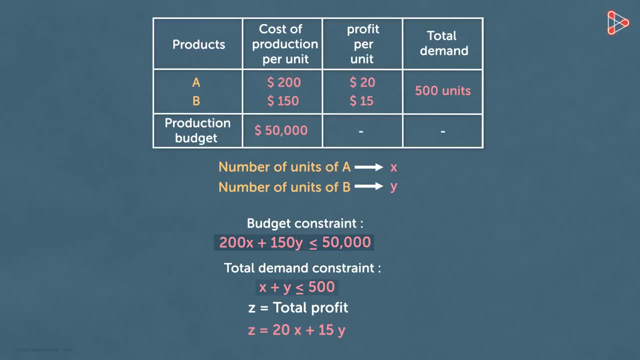 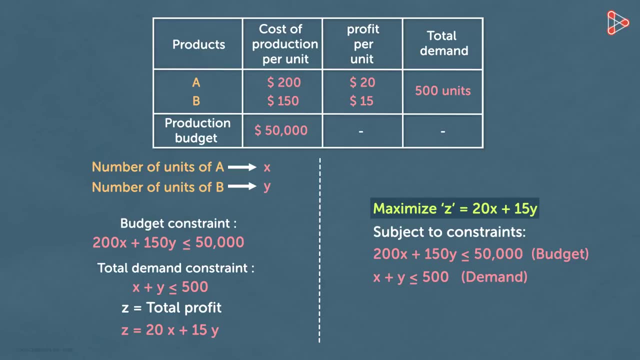 A budget constraint and a demand constraint. This is how the whole problem looks in terms of mathematical expressions. This is the objective function, and these are the two constraints. There is just one thing we need to know here, And for that I want you to answer a question. 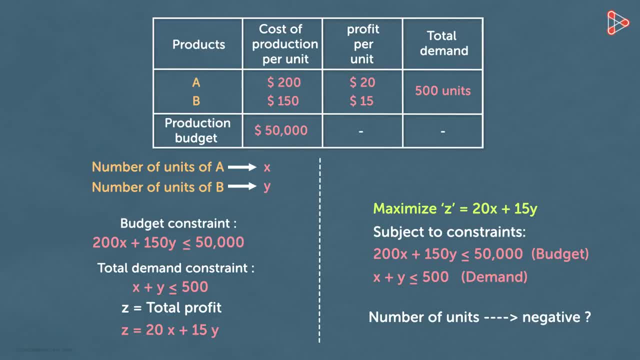 Can the number of units produced by a company be negative? You're right, it can never be negative. So we need to add the non-negative constraints. It can be written mathematically like this: It's very important to write the non-negative. 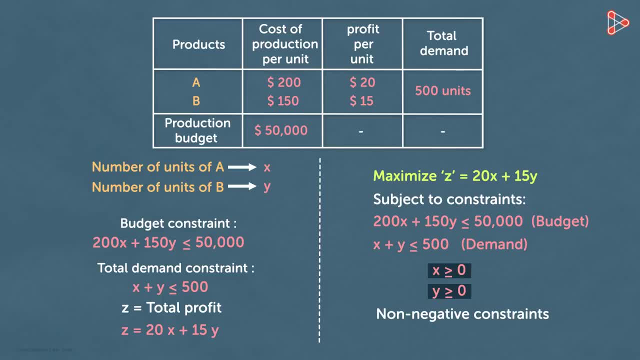 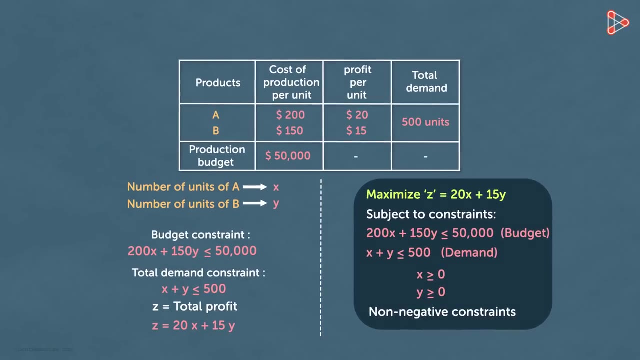 constraints in the formulation of a linear programming problem. Did you notice what we did? The entire problem of so many words is reduced to the simple format using mathematical language. As the problem is formulated in the linear form, it's called as linear programming.